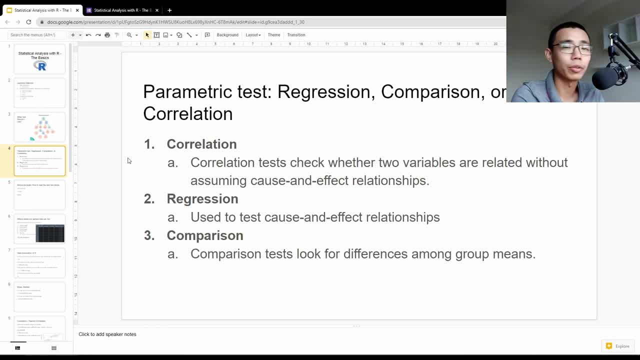 be talking about what is a parametric test, regression, comparison or correlation. So if you're not familiar with what is parametric versus non-parametric, a non-parametric test are usually data that are not very clean, like a small set of data, basically like social research science data. 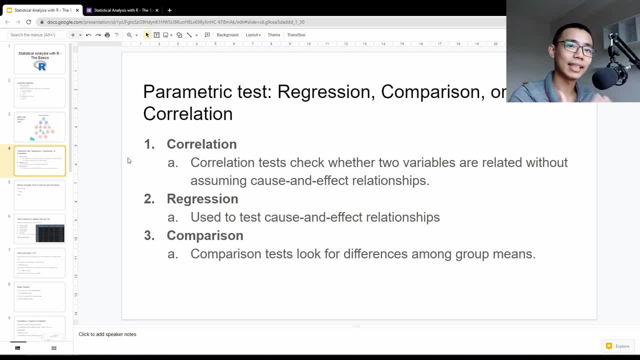 like wage income data, data that doesn't actually follow a certain normal distribution, So they're strongly skewed to one side or another or it's just very messy data. So those who are familiar with what is parametric, what is non-parametric, what is non-parametric: 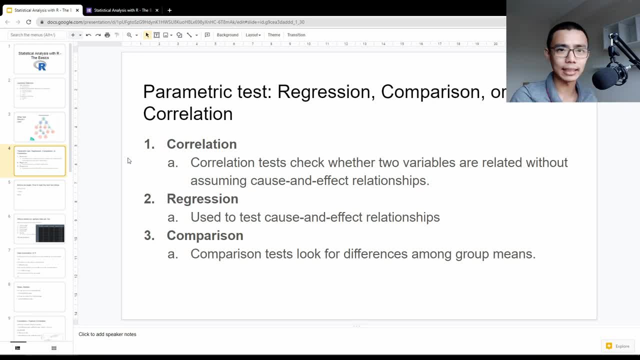 can just enjoy watching. So in this video we are going to talk about what we call non-parametric tests. So non-parametric test is not as strong in terms of the conclusion and concluding power compared to parametric. So we're not going to talk about those tests today. We're just going to assume. 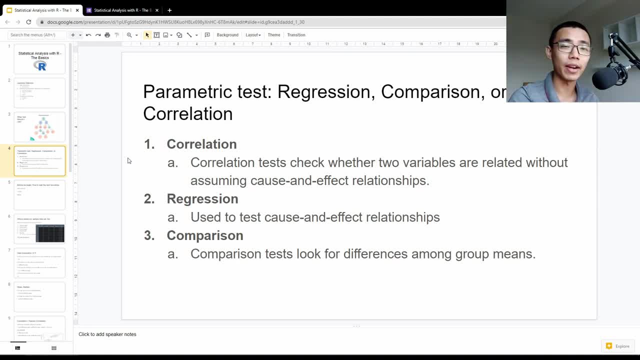 that the world is ideal, the world is great, and your data comes in a very nicely distributed format and we have a large amount of them. So that's why we are talking about regression, comparison and correlation. So what are they individually? So correlation is to check whether two variables are related, So without assuming that we have an individual relationship. So the correlation is the data that comes together, the data that comes together whatever we have, And the regression is the verification of the data and the correlation is the correlation. So, whether the 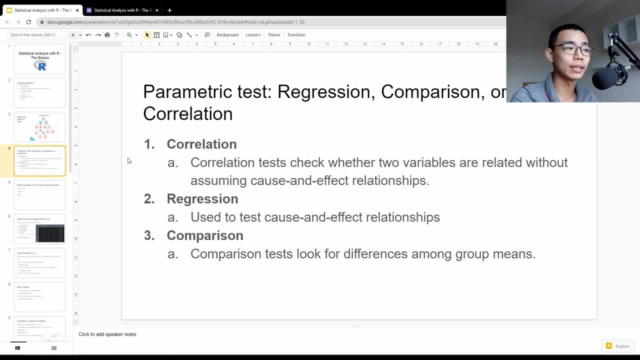 cost and effect relationship, while regression is used to test for cost and effect relationship, and the main difference between the two of them is that correlations simply tell you whether they're correlated or not, but regression analysis is able to come up with a model or an equation that you can use for the prediction if you have new data coming in. so it's a little bit stronger. 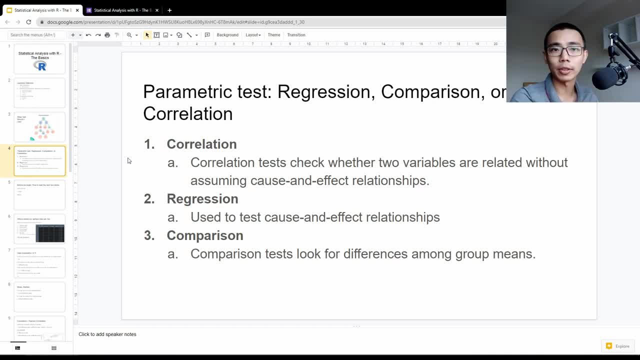 in terms of relation and regression. so the third one, of course, is comparison, which is pretty straightforward. so the most famous one is called a student t-test, where i'm not too sure about the origin, but how i understand it is that you have two classes and they both take the same exam. 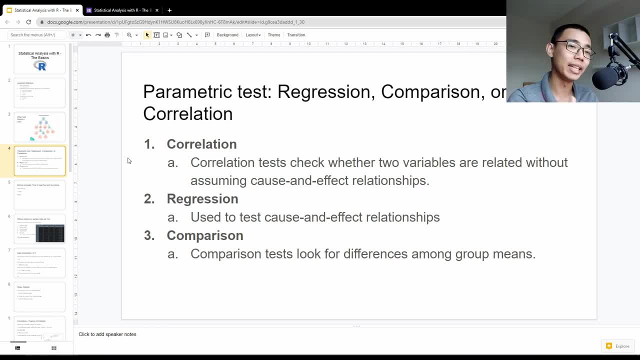 are there. significantly, are the means of the two classes significantly different from each other, which is why it's also very commonly called a student t-test. i'm not sure that's the origin, though, so don't quote me on that. so before we go to r, so just to make sure that you are able to. 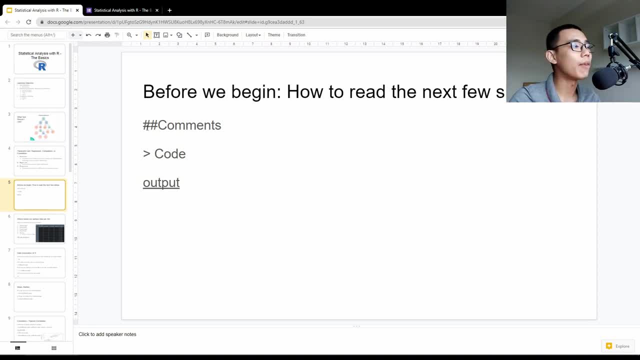 understand the way that i write my google slides and everything that comes with everything that i include in the latest slides. if there's two hashtags, sign in front of it. it's a command. so these are just something that i wrote. do not run it. it will not run. 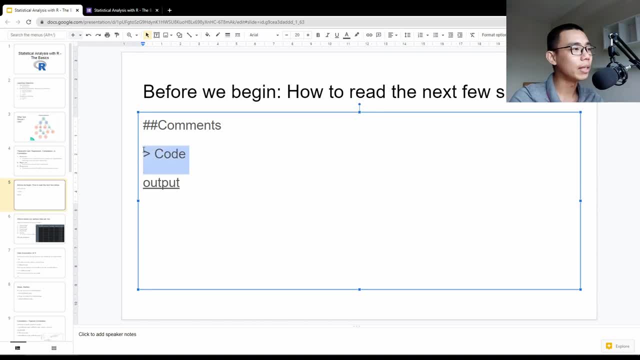 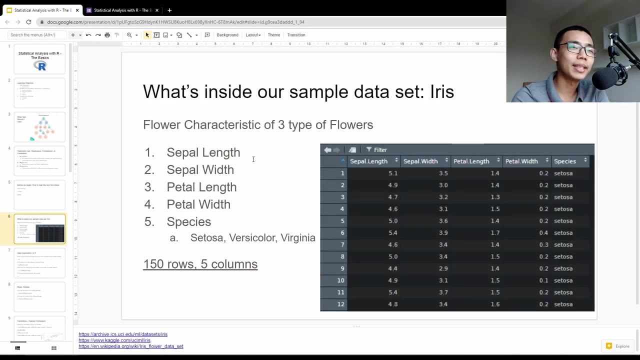 it will not run in our environment. everything that preceded by a larger than is the code. that's the actual code that you want to copy into the our environment. lastly, the other lines you should output. and before we start again, let's look into our data set. so we're gonna again use rs data set. 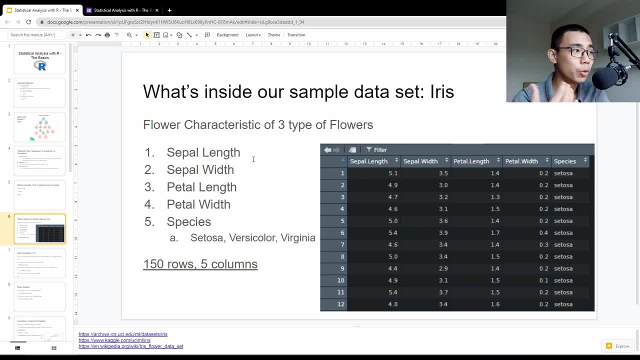 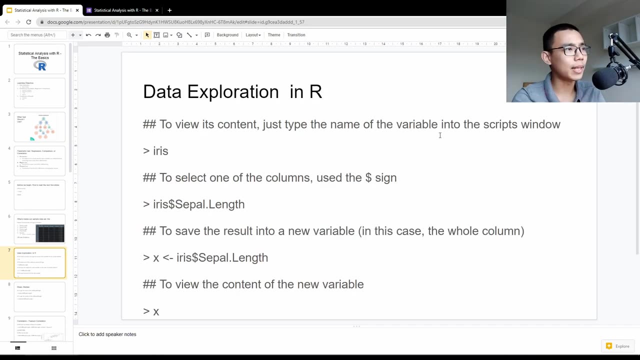 it's very famous, very popular and they've been used everywhere. so we have a characteristic of three different flowers: uh, centosa, versicola and virginica. and we have several lines up with petal and petal waves and three species of flower, 150 of them. four type characteristics: okay, so first one data explorer. 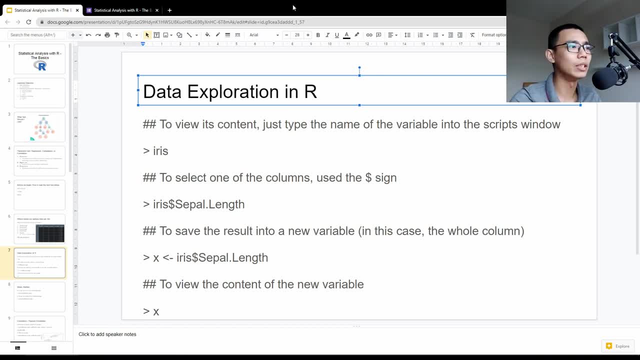 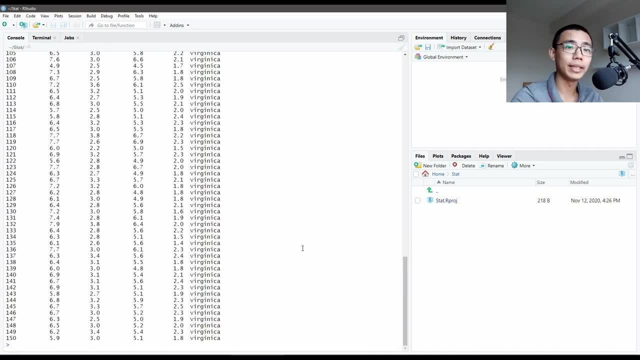 now. so how do i import the iris data set into r? uh, very straightforward. when you open r, it looks like that. what you do is just type iris and press enter, and you'll be greeted by the five column that we have showed you just now, as well as the species. okay, so what i usually like to do is to pipe the iris data data. 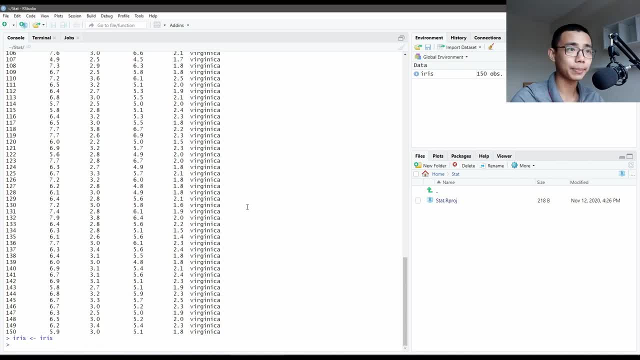 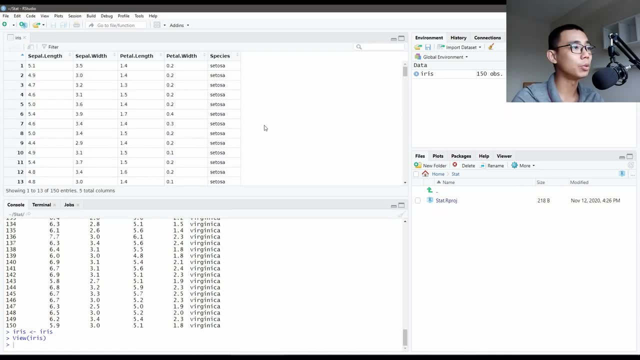 frame into a new object called iris. so in this case it allows me to see a value on object, a data, here in a global environment, and when i click on it i'm able to have a spreadsheet view of them on top so i can have a a clear idea of how it looks like. when i'm trying to code, i'm trying 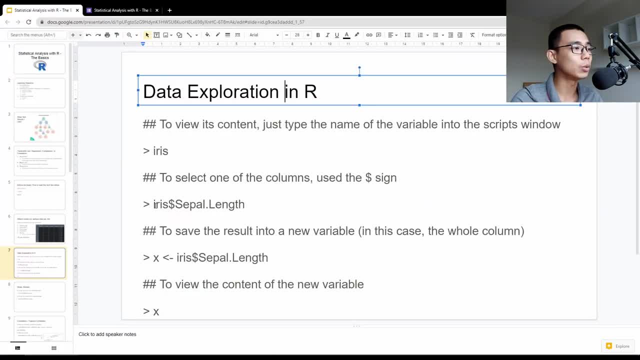 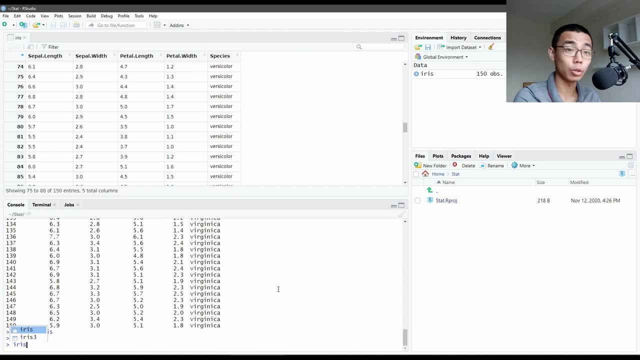 to do things in my console. okay, so the second one is the data set, and we are just bringing in the data set is to select one of the column. So we use the dollar sign, fairly straightforward. So you just type iris in your console window. 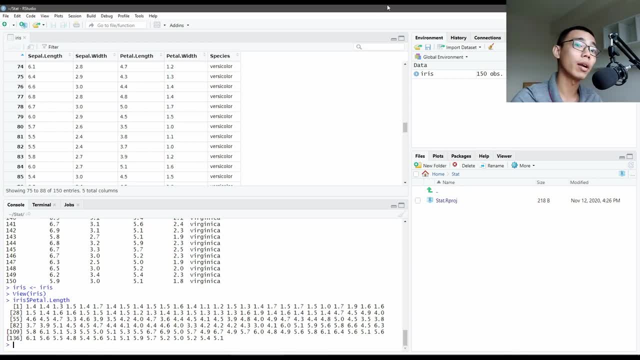 select the dollar sign and go to pedaling, and that is where you get 150 value over there. So you can also do that by piping the data into a new. well, I shouldn't call it piping. We are assigning the due data into a new variable. 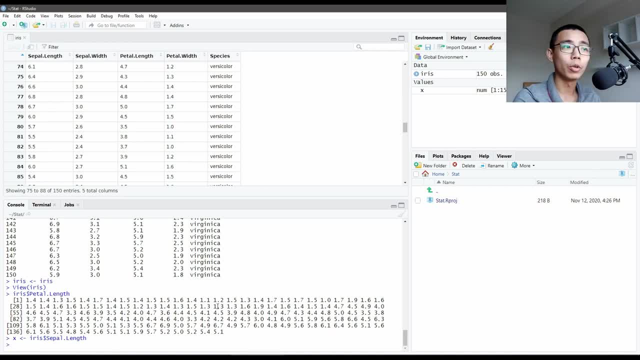 called x over here. When you run it it won't show any output, but on top of the global environment here it will actually show you a value called x with 150 different numbers. So these numbers are the 150 pedal sepal length. 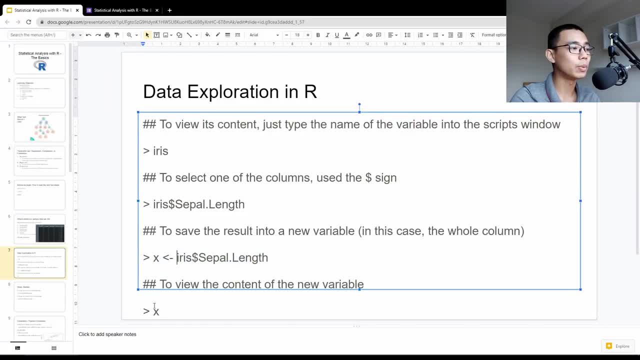 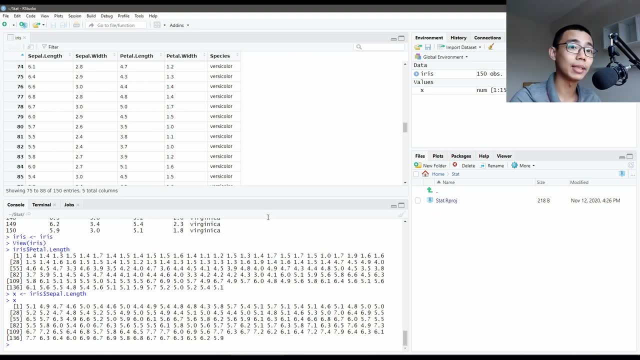 that we have selected earlier and being assigned to x. So once we've done that, we can also just type x, press enter and be able to view the 150 different values that we just assigned to. Okay, so once that's done, 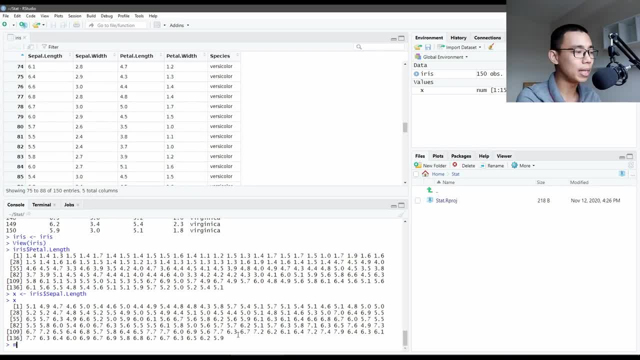 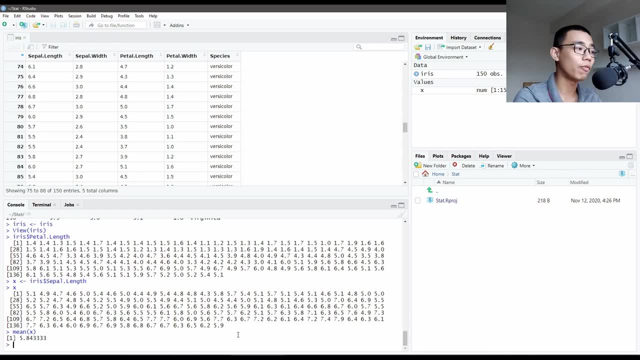 let's go into mean and median. So how do you run the mean and median? It's pretty straightforward. So the mean of x: just type mean open bracket, close bracket and put x in the middle, enter. you've got 5.833.. 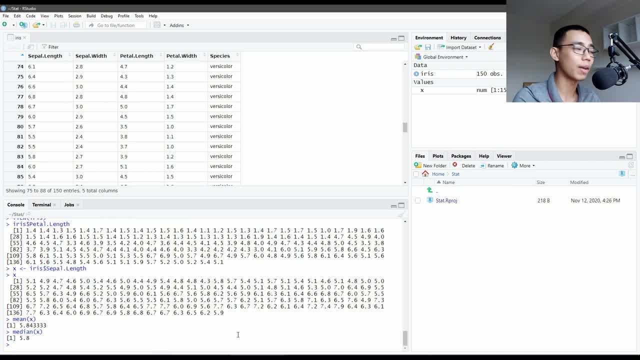 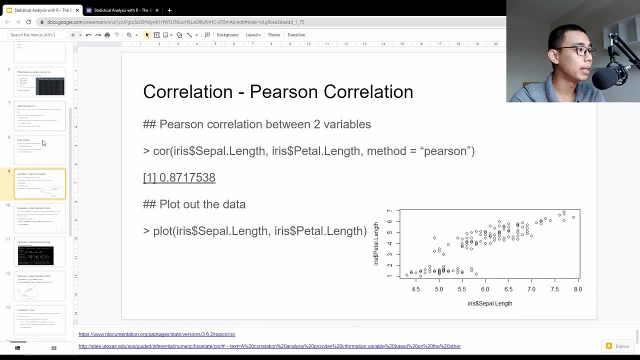 And if you want to run the median, just type median and x. you've got 5.8.. So all these are pretty straightforward. Okay, so the next one is correlation. So how do you run Pearson correlation? It's again pretty straightforward. 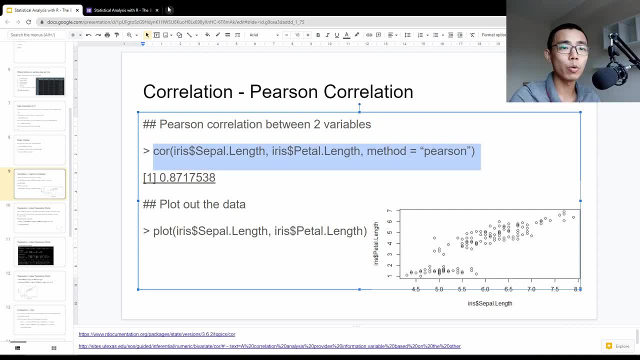 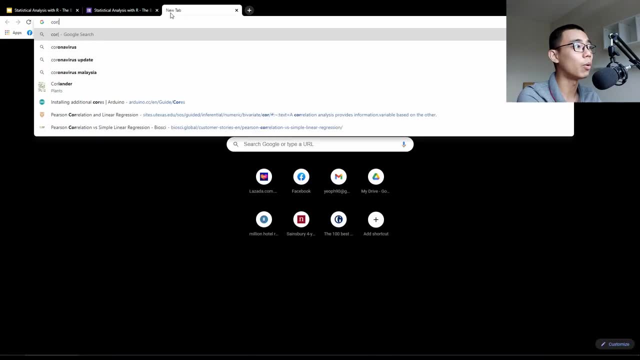 The function is called COR And for those that are new to the R environment, what you can do is that if you want to know more about a certain function, you can just type COR and then just type R, And this guy goes right back to documentation. 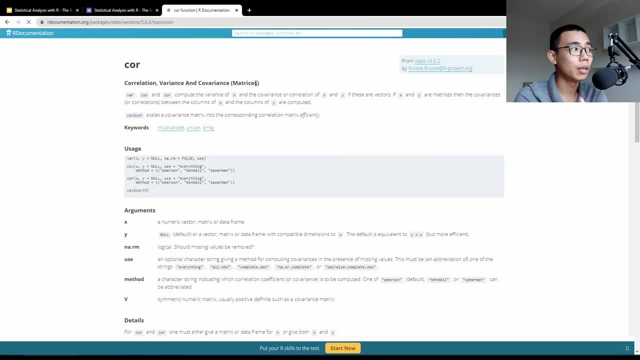 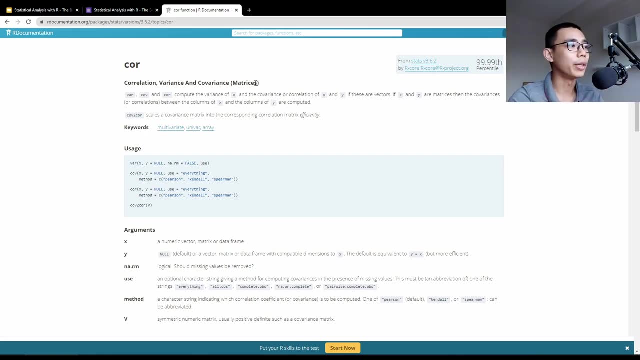 Okay, so this will have the official documentation from the R, no, the CRAN, the comprehensive R archive network, the CRAN- basically showing you that what do they do and what kind of things you can change. Okay, So I'm going to go ahead and run this. 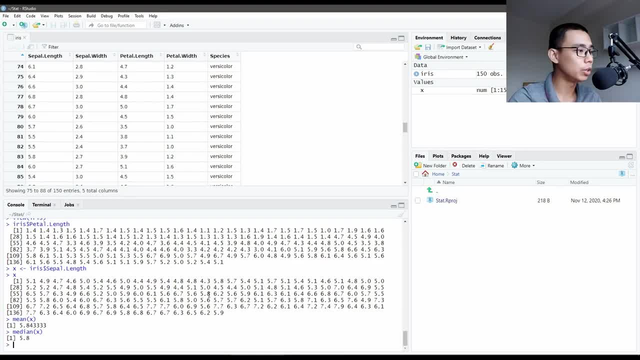 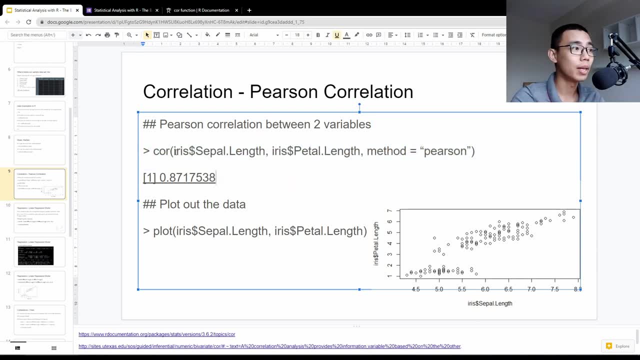 I'm going to leave yourself to read more into that. So what we usually do is to just go back to the slide, copy the whole thing And this: we are comparing the two different data set from simple length compared to the paddle length. 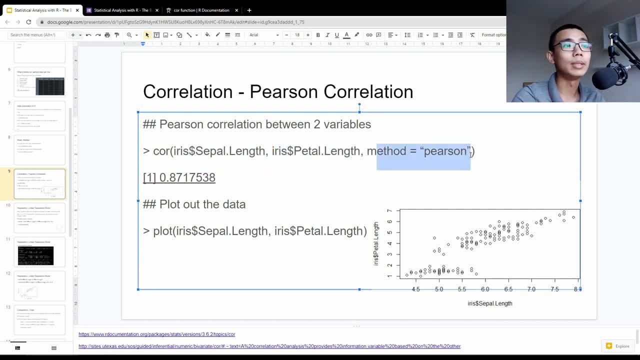 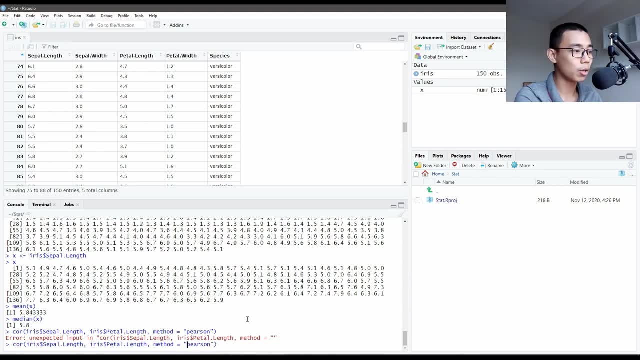 And we want to see if they are correlated in a certain way. using Pearson method. Okay, just press it. And, sorry, you might have to change the double quote here, because I don't know why it's some encoding issue that doesn't recognize. 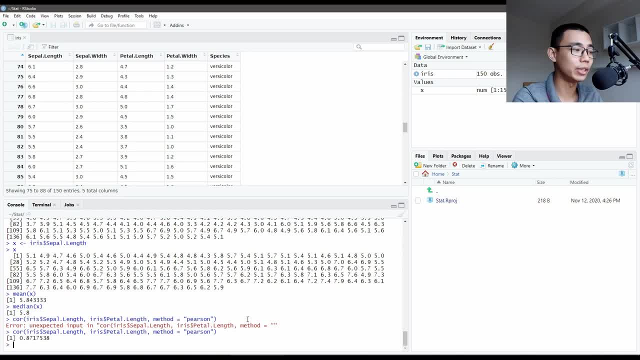 But the output, which is 0.8717538.. So what this means is that everything closer to one means that strongly correlated positively, and being near to negative one that's negatively correlated, but then strongly negatively correlated, negatively strongly correlated. They're one of them. 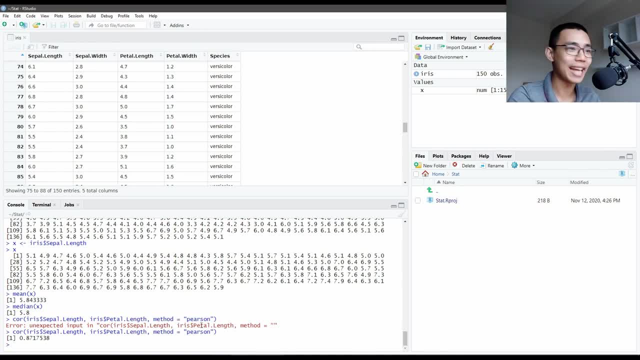 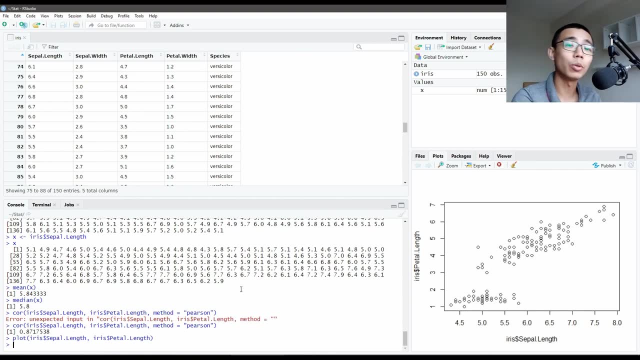 And everything close to zero means they're not very correlated at all. Okay, So what you also want to do, instead of actually just get the 0.87, and call it a day, is also plot out the data and understand that. Does it look like a correlated data or not? 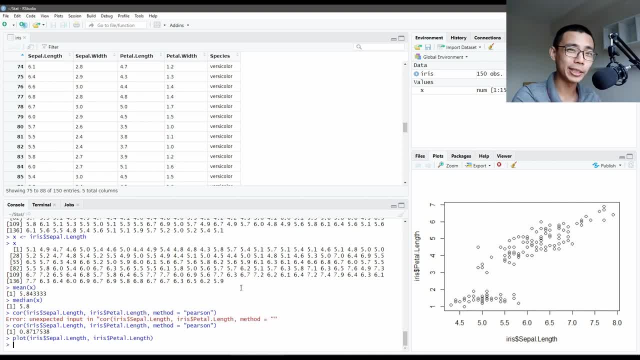 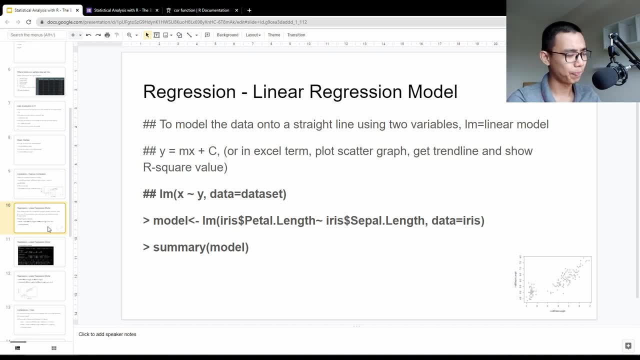 Then this will be able to tell you. Remember, there's also three species here, So most likely they would be correlated, but not that much. Okay, so interspecies maybe. So next one we're going to do is after we've finished. 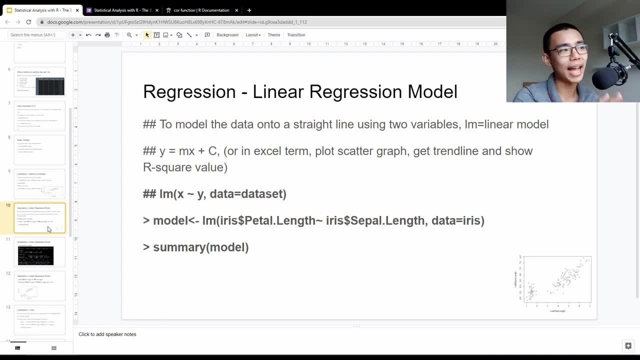 done the correlation. we want to create a linear model because the model kind of looks like a linear relationship, not a log, not an exponential. So we want to run a linear model. So the equation for linear model is just: Lm, x, y. data equals to dataset. 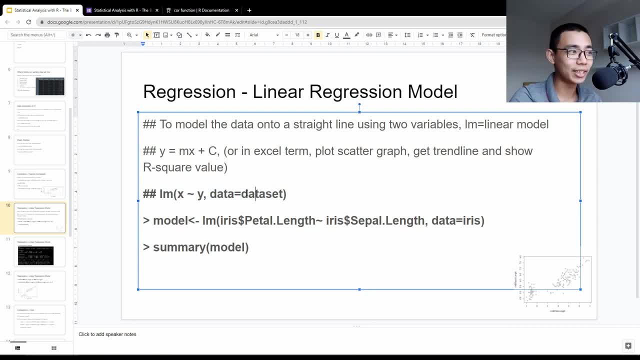 Okay, So data equals. don't change that, Only change the name of the dataset to your dataset. So I've included an example over here When model is assigned as Lm petal length to sepal length. So we want to compare the relationship. 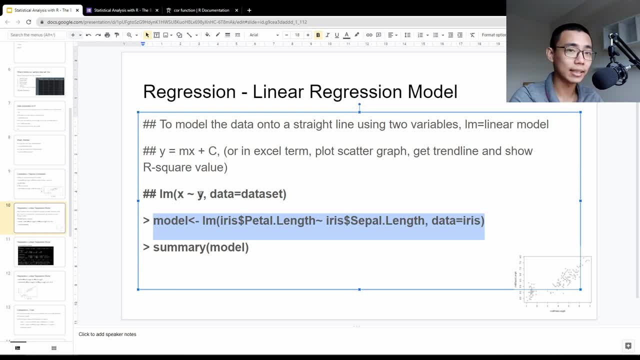 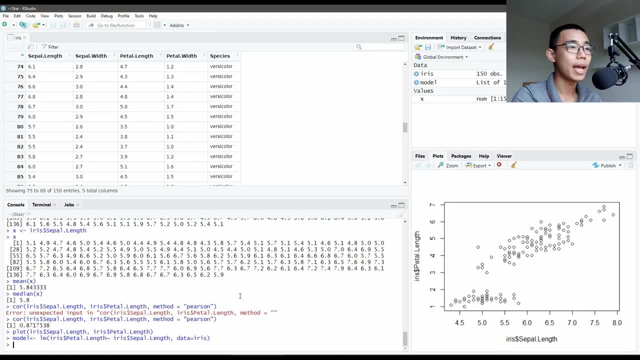 between petal length and sepal length. Remember, R exists, y exists in the back and data is equal to the iris data that we run just now. So what we do is that we copy paste this in and you will actually see a new object called model. 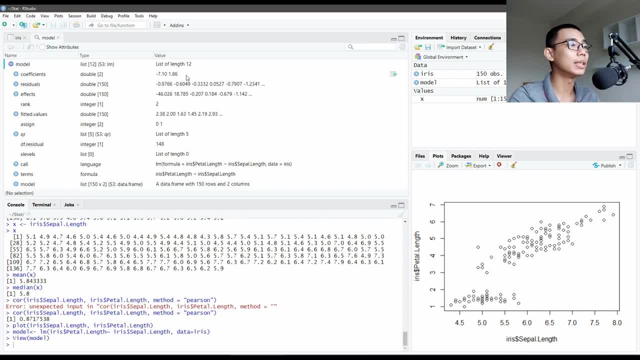 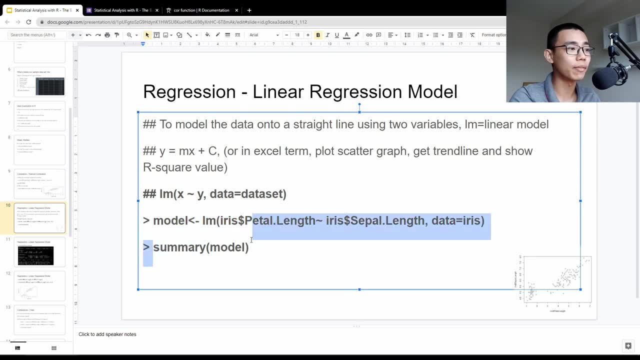 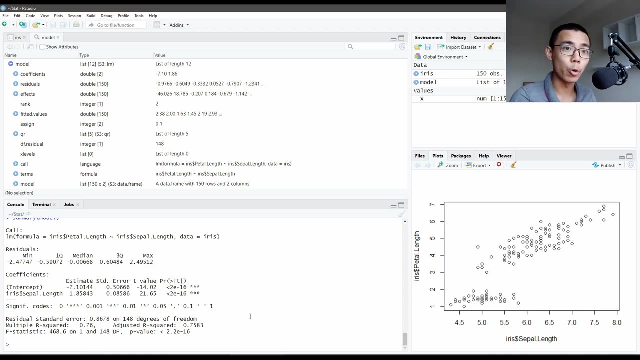 which is a list of 12. You can actually click in and you can see all the individual breakdown of the model. So just to get a more simple idea of what it is, you can actually use another function called a summary function, And this will actually just give you a more simplified output. 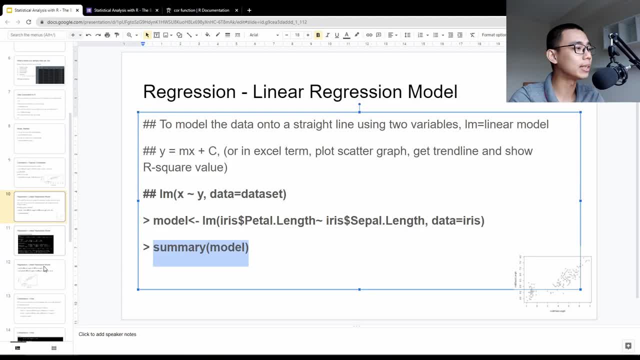 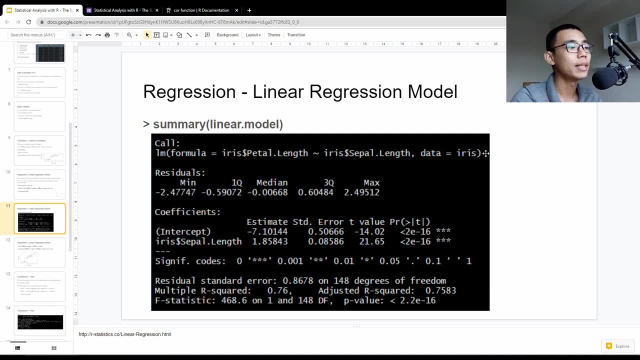 of the summary of the analysis. Okay, So let's look into this analysis a little bit over here So you can see that we can actually see our formula that we used previously and we can actually see the residual coefficients, significant codes, which is whether it's significant or not. 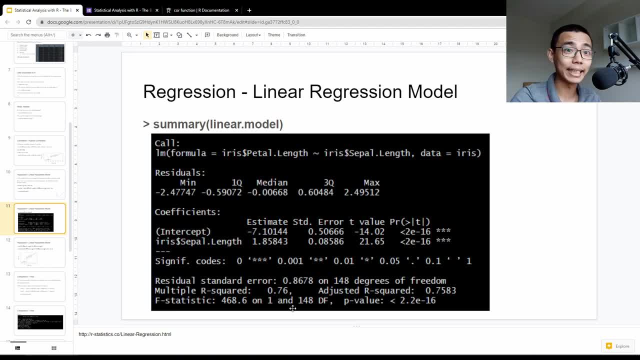 And we can see all the individual details that we want to look at here. So there's something that I actually just realized is: what is the meaning of the? what is that? where is the thing that I'm trying to say? P- oh yeah, there's a R-square value and a P value. 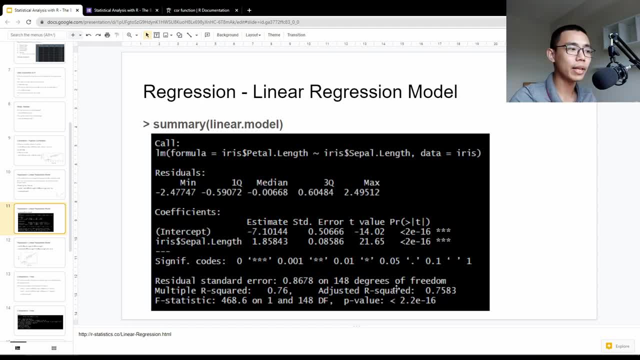 So the difference between R-square value and P value is that R-square value actually measure how far the data is from the line that you draw, while P value justify how generalization generalizable your data is to the populations. Okay, So if you don't really get what I'm trying to say, 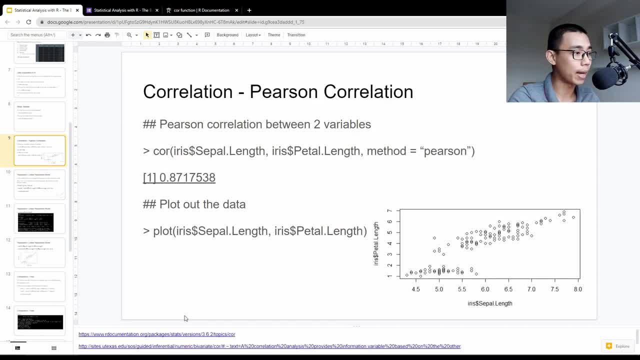 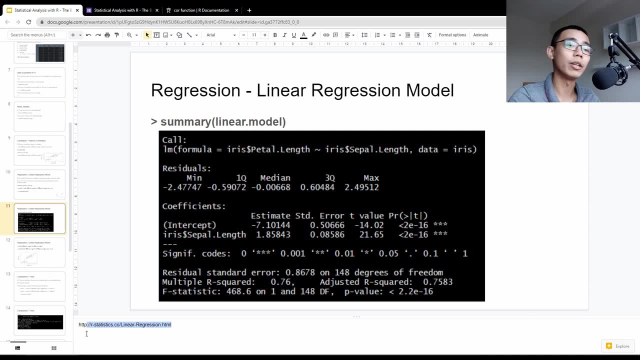 you can actually read from the field where data include yeah here. So you can actually read about the correlation here in the notes, in the slides, And you can also read about the linear correlation here where I include it in the slides. 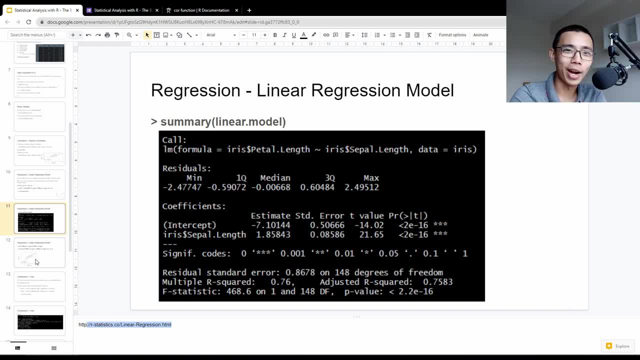 It's a bit. you know, I don't want to make this video another a one hour video again, So maybe we'll come back to this when we have more time. So, but basically that is how you run a linear reaction model very easily. 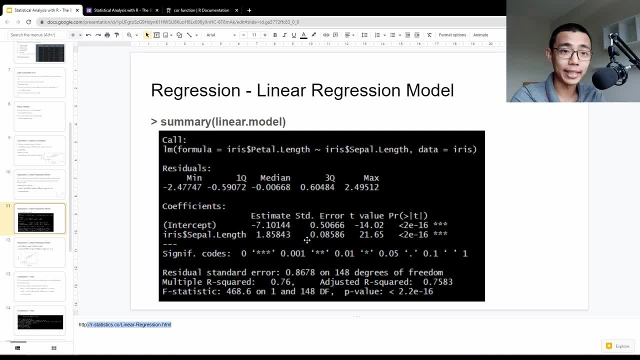 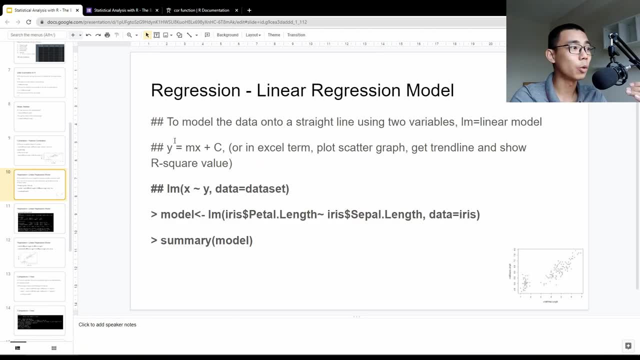 And you can get your intercept and you can get your your gradient. Okay, So you can get the intercept in here and that's your M and C. where is it M and C here? So Y equals M, X plus C. your gradient is your M and C is your intercept. 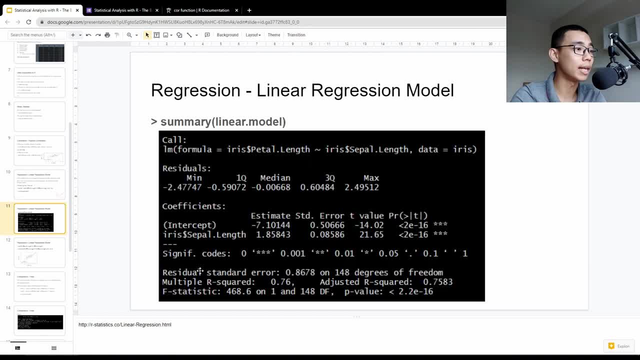 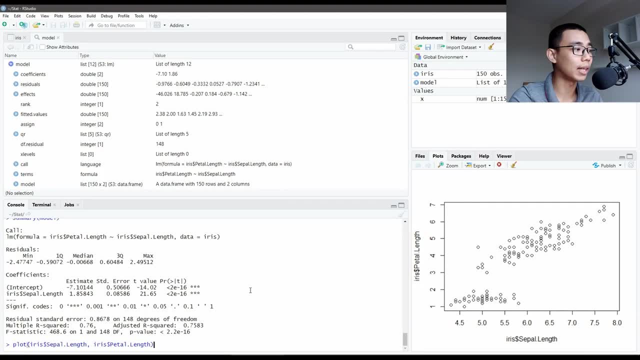 So you can actually get your linear model quite easily based on the summary that output that you got just now. Okay, So it's also generalized. It's also advisable to try to plot the lineup just to check if you know the concept is correct. 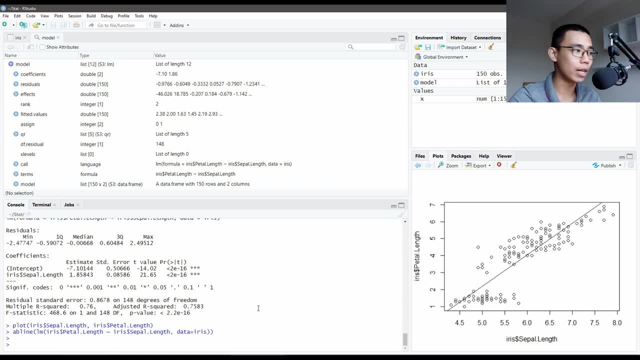 where we have slightly low R square value. Our R square value is only around here- 75% or 76% with our adjustment- but our P value is quite high. As you can see, both of the data is not actually very near to the line. 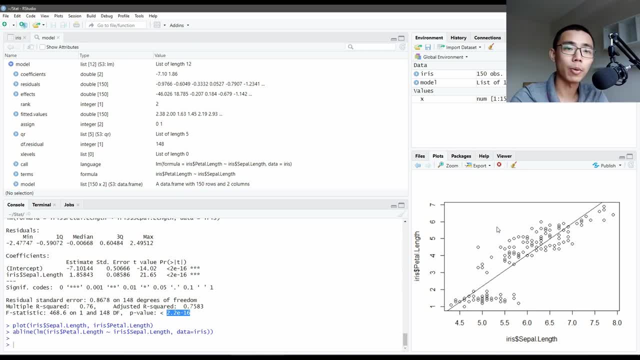 which is why we only get about a 75% of our square value. Okay, So that's basically linear model And you can see that the intercept is actually minus seven, which is not drawn here, And our gradient is 1.85.. 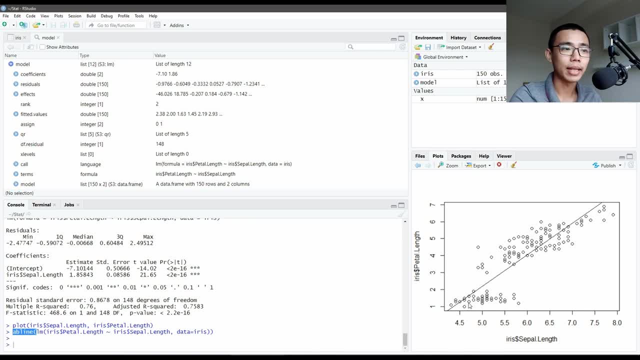 And if you don't understand why it's F line. F line is just the way that how we draw the, the linear line over here. Okay, So let's just try that again When we plot. it would not. it will show a plot without line. 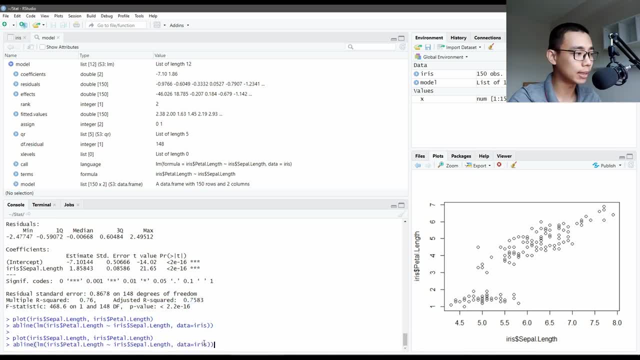 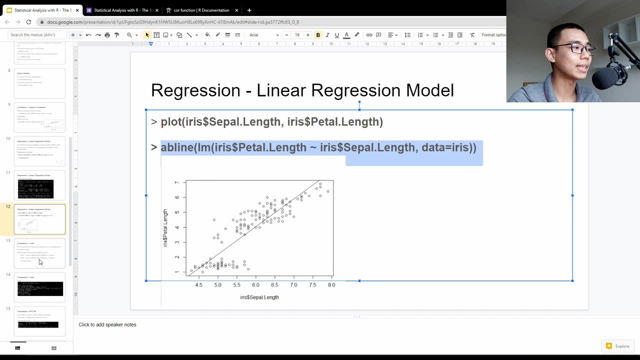 but when you actually run app line based again based on this linear model, it actually draw your linear model directly out on the plot. So that's make it easier to understand what we're trying, what we're actually trying to do. So let's move on to our third agenda. 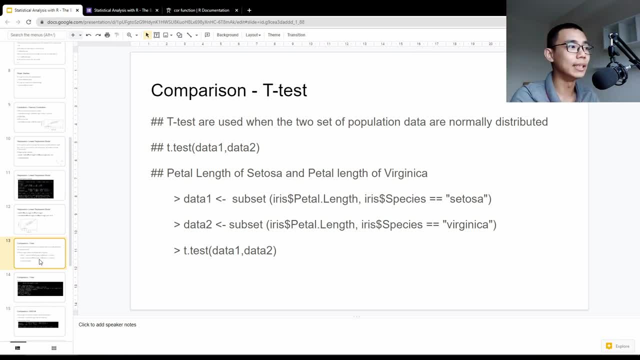 which is comparing a t-test. how to run a t-test into in R? Again, very straightforward, just t-test, data one and data two And, of course, the. the problem is that, how do you prepare data one and data two? Because, first of all, 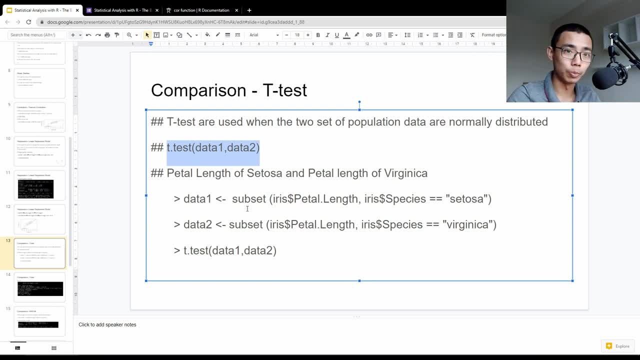 you don't understand. t-test compare data in different groups. So what we need to do here is to separate data one to only contain Centosa flower and the data two only contains a Virginica flowers. So what we do here is use a equation called subset. 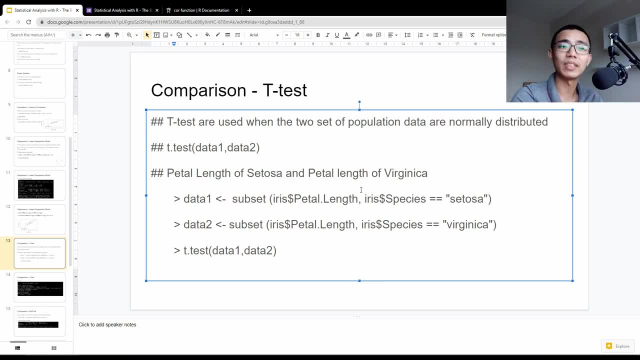 which is able to select only the first, not, yeah, the first field, which is only select the data where where the flower species equals Centosa, And subsequently we're doing it for data two, which only select flower with the species Virginica. 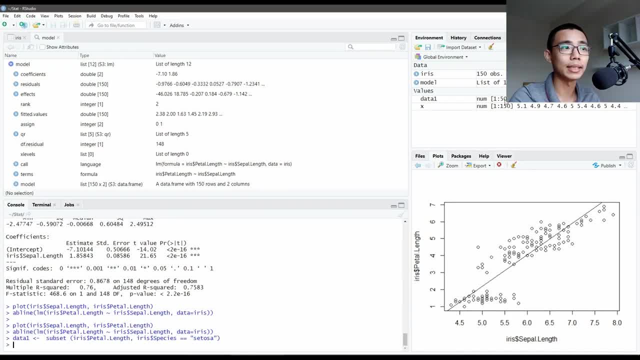 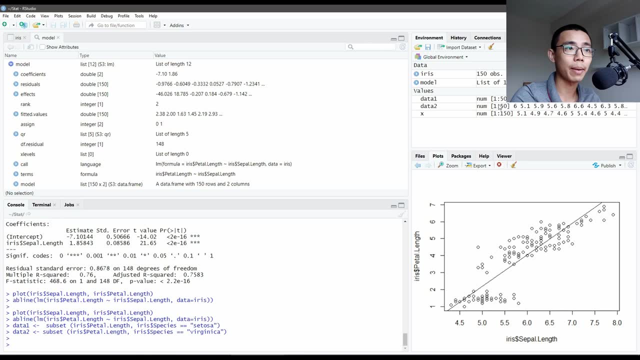 Okay, So let's just copy this and we get our data one here. as you can see, there's 50 of them and data two. we actually can again select data two and you can ensure data is correct by looking at here. 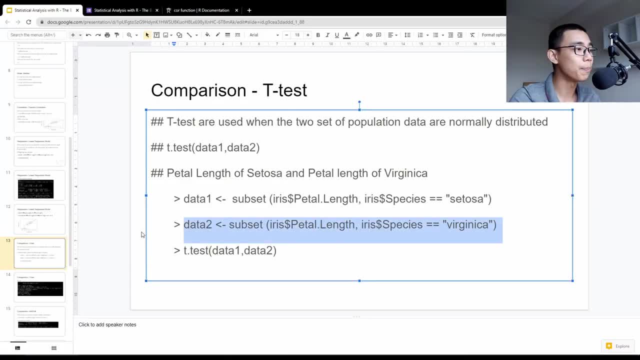 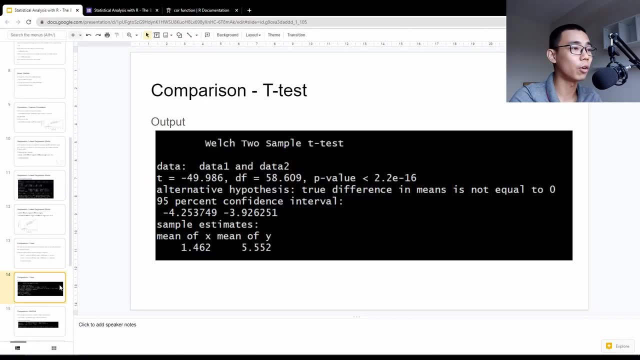 or if you want to visualize data again, you can also type it in quite easily And we run a t-test on two data like that. Okay, So this is a Welsh t-test. So let's go back to our slide for the example here: 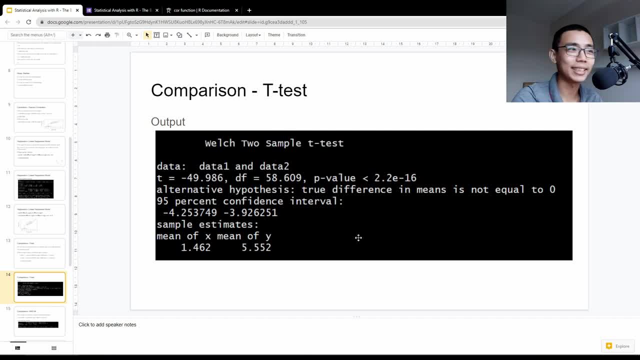 So this is a Welsh two sample t-test And the most important things about the t-test is to just look at the p-value, And our p-value is actually quite low. It's actually 2.2 to the power of 960.. 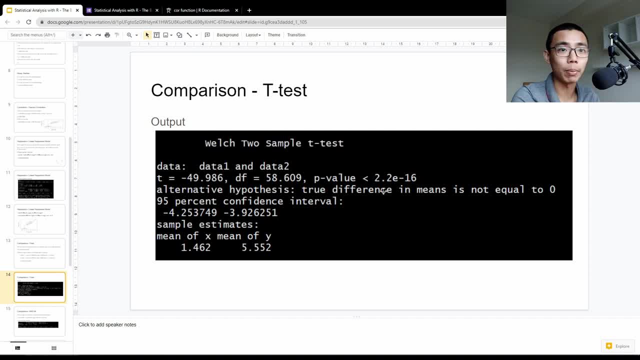 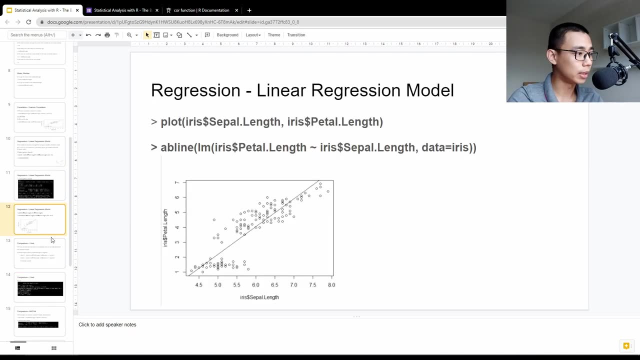 So we can actually quite confidently tell that these two sample has a significant difference in their petal length. And that's basically, and this is your confidence interval And with your with 95% confidence. So again you can find the notes into our notes in the 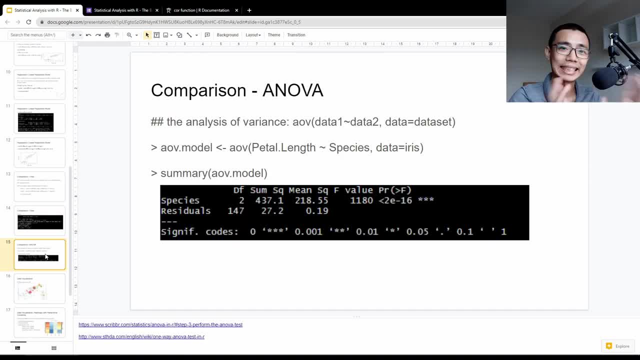 I'll add more description about what is t-test in the Google slides later. You can find it down there when you go and click on it. Okay, So the next one is actually ANOVA. So people always ask: what is the difference between ANOVA and t-test? 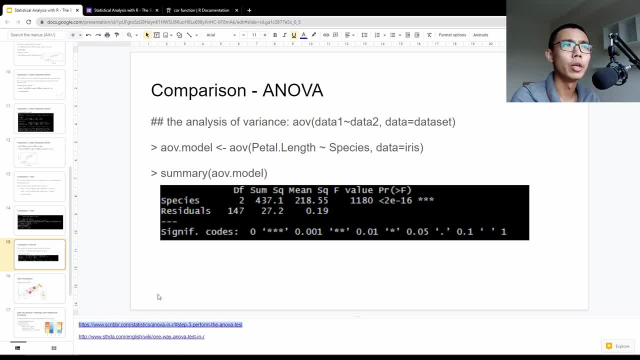 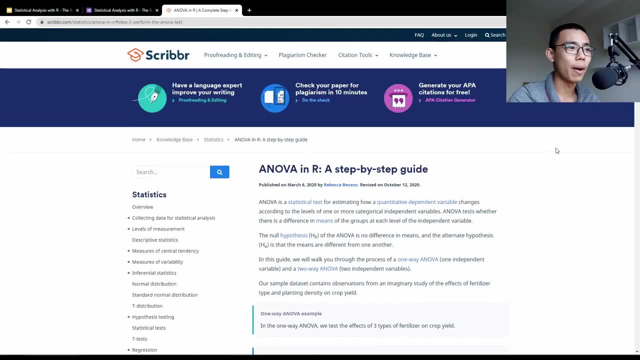 And to put it simply, ANOVA is able to run more than two sample sets. Again, it's a massive, massive. what is that called? A massive simplification, And if you do want to know more about what's the difference between ANOVA and t-test. 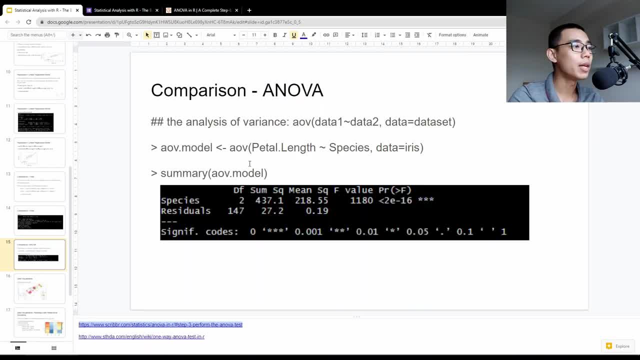 you can actually have go to this website over here Scribble. I don't want to put too much, otherwise there will copyright strike me or something. But I will put a link in the Google slide over here. Please do go and have a look on. what is the difference. 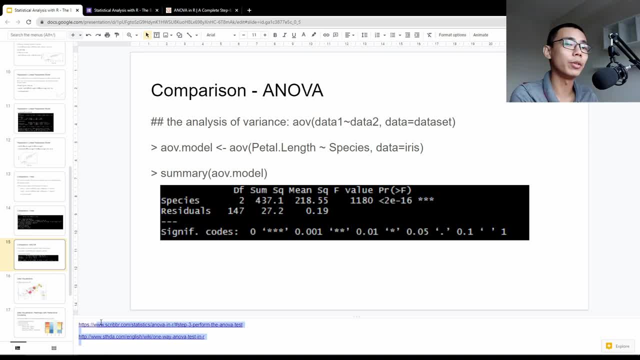 between one-way ANOVA, two-way ANOVA, and how, when to use t-test and when to use ANOVA. So to actually run ANOVA, we're going to use a function called AOV, which is actually analysis of variance. 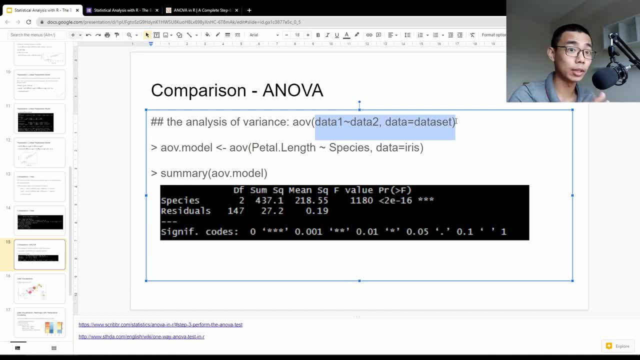 And the data structure is similar to the linear model that we run just now, which is data one to data two and with data is equal to data set. So what we tend to do usually is to again run the function and pipe. 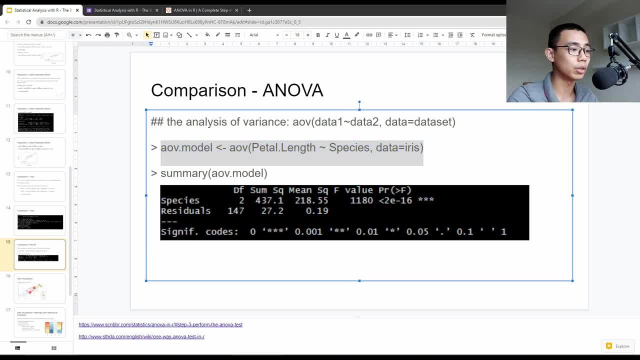 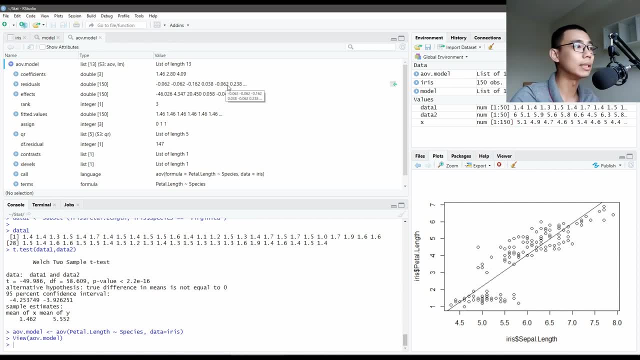 and assign it to a new object called AOV model. So we can do that and we can see your model showing up as a list of 13, with all the individual calculated parameters here, And what we can do is that again. 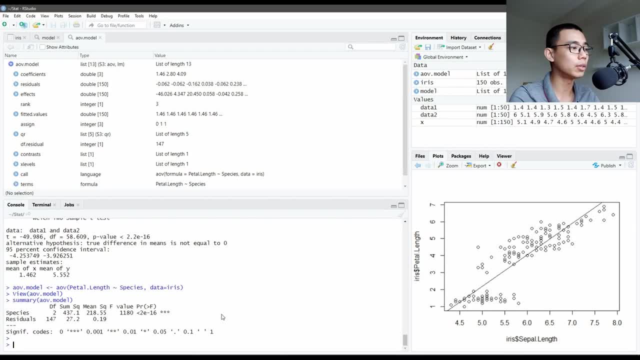 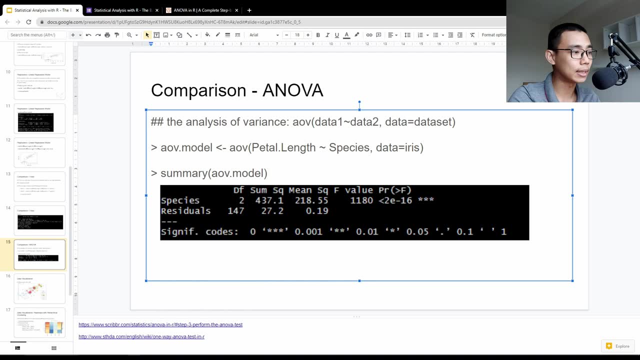 we use the same method, which is summary AOV model, And this will give you the significant level, the comparison between two groups. Okay, so you can see, this is the same things that we are running just now. So we have species. 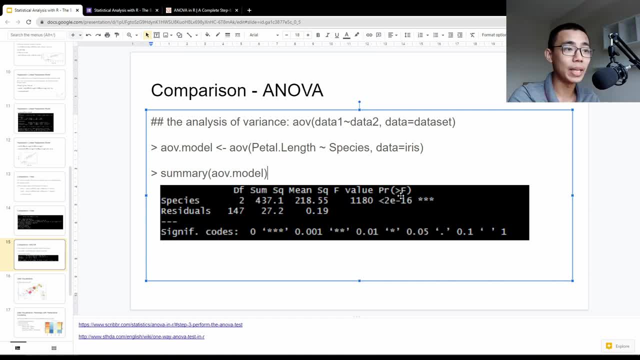 the degree of freedom is two, And again we are looking at our P value, which is minus two to the power of 16.. And you have three S-Rig over here means our confidence level, that these two groups of data is significantly different from each other, is 0.001.. 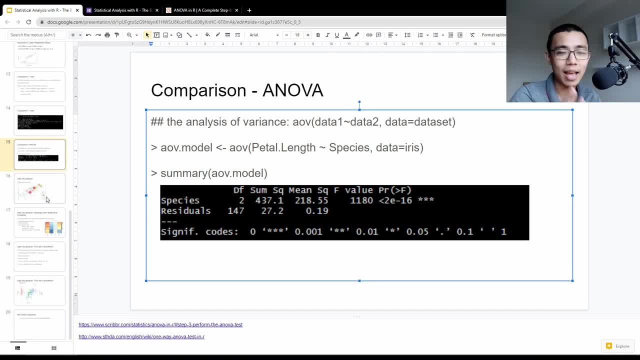 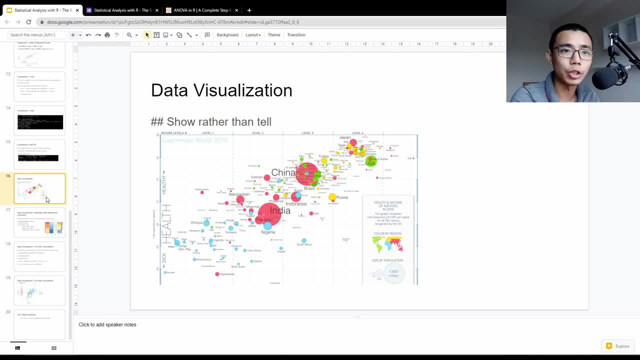 So we're quite confident that this would never happen by chance. Okay, so we have done all this thing. It's actually very important to understand a little bit about data visualization because, to be honest, this is not interesting. You know, people look at this data. 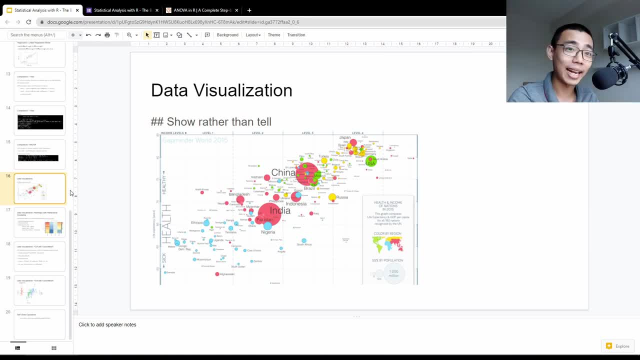 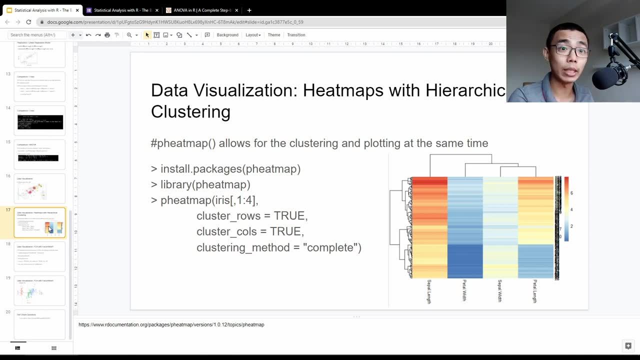 it tends to get a bit tiring when you are looking at data tables all day. People like to look at figures and so on, And I believe heatmap is one of the really easy way to do it And you are able to show a lot of information very. 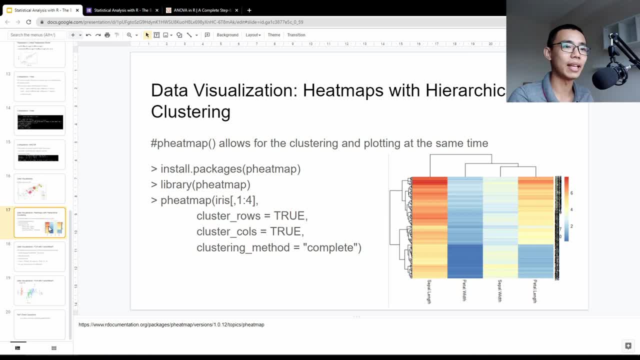 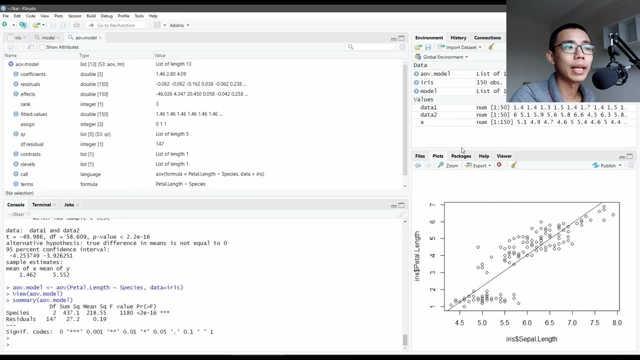 very fast and very, very easily because it has multiple dimensions on it. Okay, so we're using something called heatmap library. So how do you install a library? is that you go to package, install and type in. pheatmap actually stands for pretty heatmap. 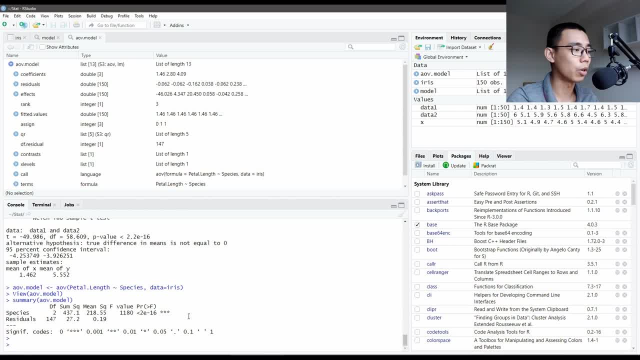 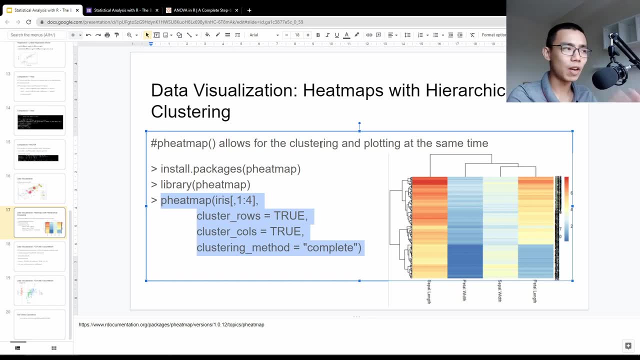 And you just press install and that will install the library into into your computer, And what we do is that we're going to run this. what is that called? This function which actually generate the heatmap that you see on the right? 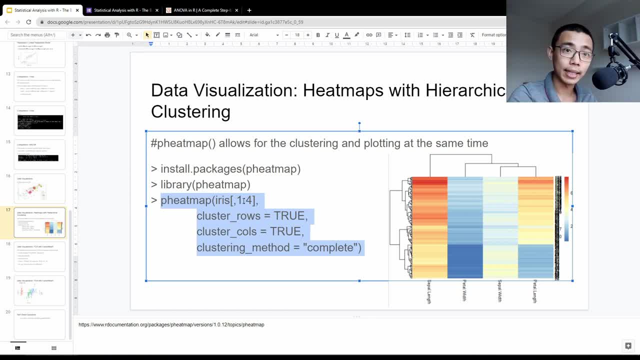 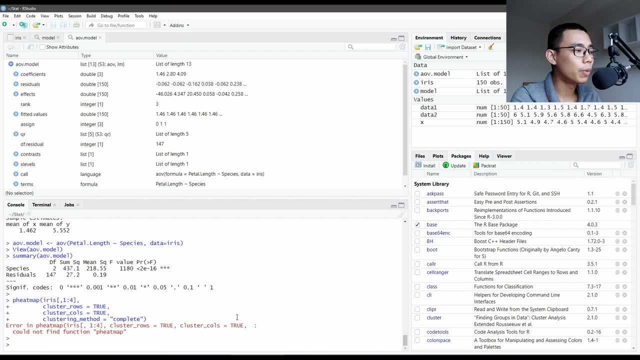 by selecting the first four columns in the iris dataset And we want to cluster the rows and cluster the column using a complete clustering method. Okay, so what does that allow? Ah, sorry, I haven't loaded into my environment. Ah, I haven't installed. 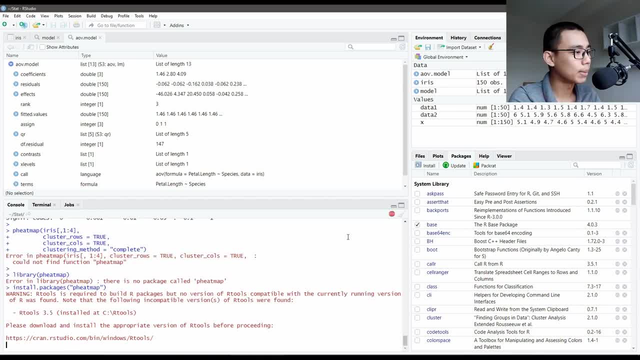 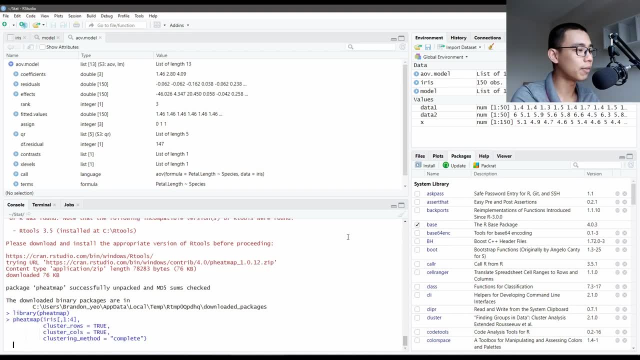 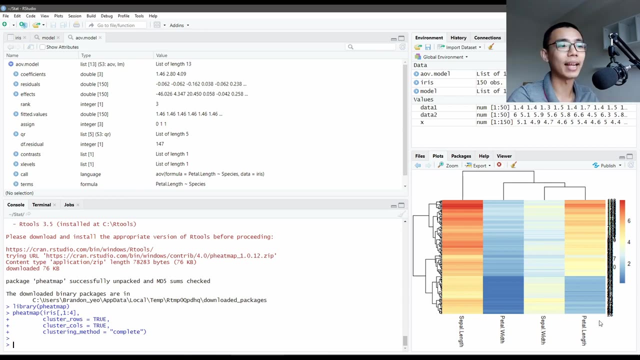 Well, the problems are multiple computers and sometimes things happens Okay. so again, run this and do an environment and we run the function again. So this will generate heatmap on the simple length, simple width, simple simple width and petal length again. 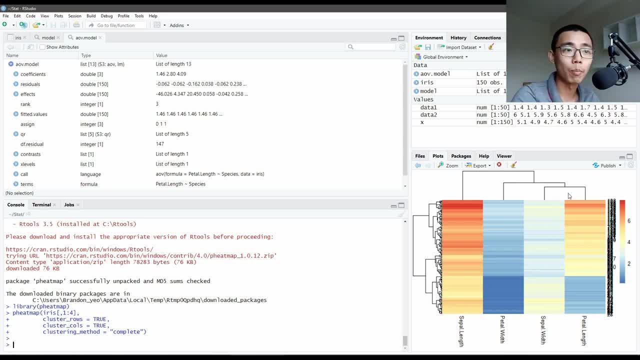 Okay, so we can see that simple width and petal length are more closely related to another in terms of their behavioral patterns, while simple length is the furthest away from all the four parameters. And you can see how the sample groups together and from one another, based on the clustering method. 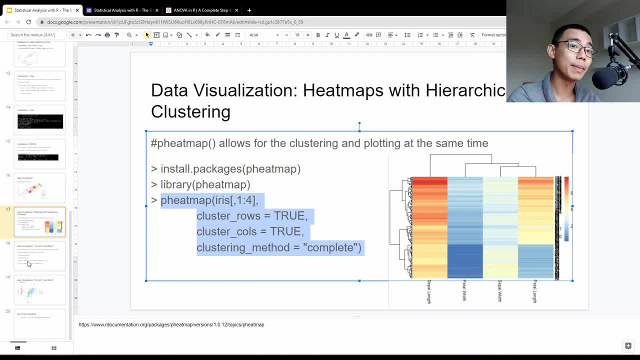 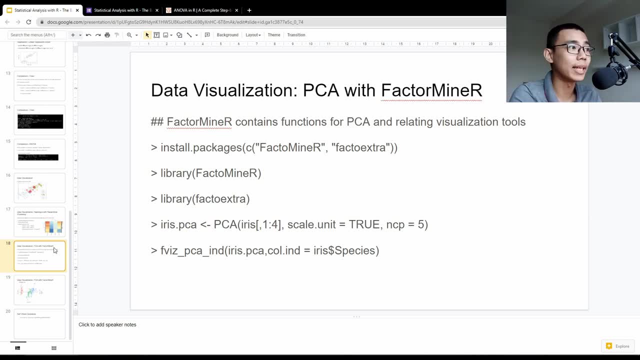 Okay, so just an example: understand when to use it and depends on the size and type of the data that you do. Okay, so the next one, the last one we're going to run today, is actually principal component analysis. Again, principal component analysis is very useful. 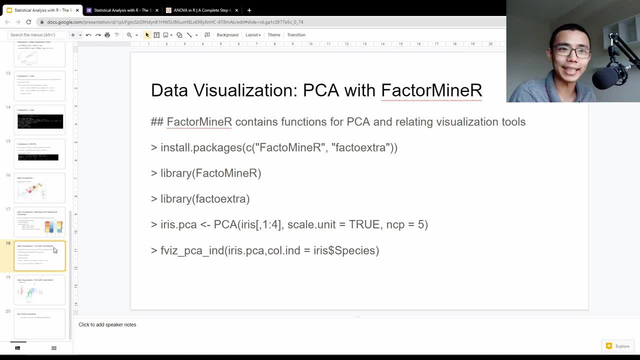 when you have multi-dimensional data- Let's say you have a 600 dimensional data, so that is data with 600 different column- You want to know which few are the most important and which few are very similar to one another. You want to throw them away before you fit. 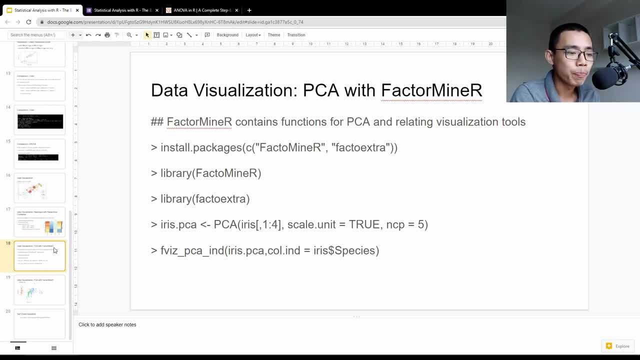 into your machine learning algorithm or you just want to know what are the most important column that I need to analyze? PCA is able to do that. Okay, so we're using two library called FactorMyR and FactorExtra, So follow the same method. 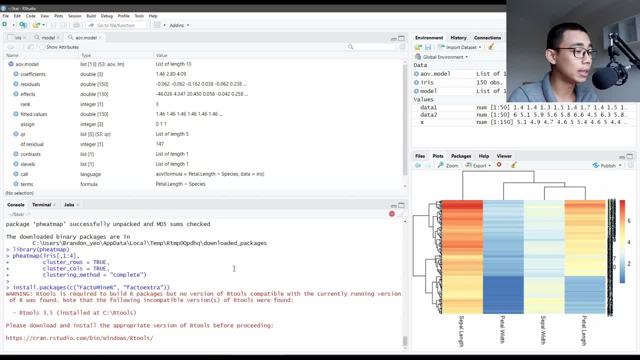 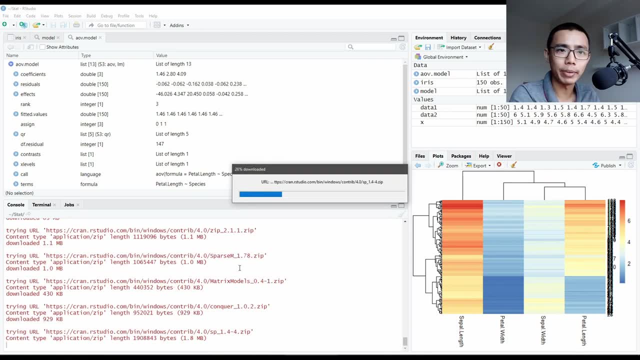 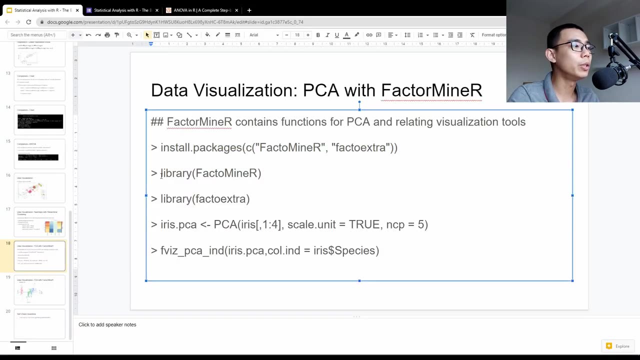 just install the library into your environment. This actually might take a while, because our FactorExtra and FactorMyR is actually a very, very big library that's actually useful in a lot of different things, rather than just PCA. Okay, so we do the same thing about library. 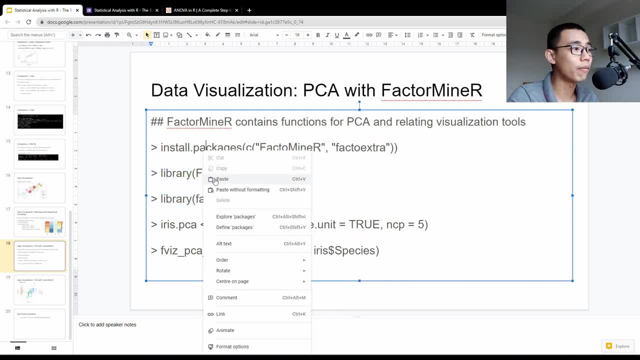 which is just load the library of FactorMyR and FactorExtra into the environment And we're able to run our PCA using a function just for PCA. Okay, again, we're just going to select only the first and then we're going to do the same thing. 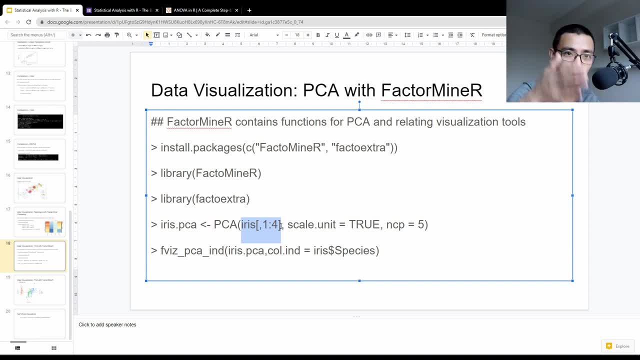 for variable, because they're numerical and everything, And the fifth column, which is species. we want to throw it away And the rest we can actually remain as default or try to change around and see what happens Again, if you need documentation. 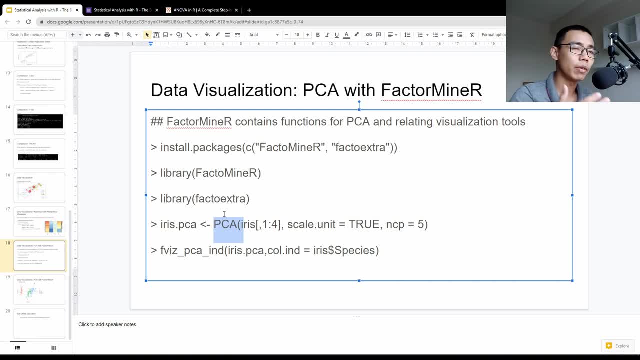 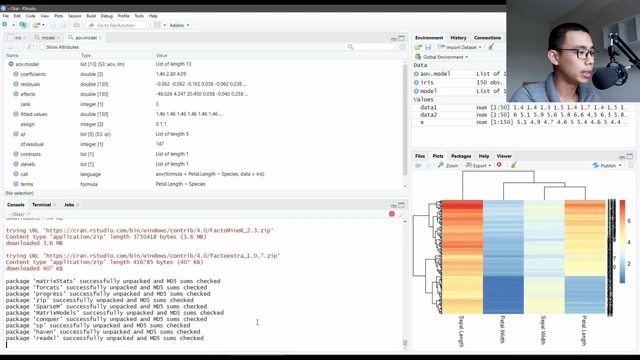 just go and type the name of the functions and just run CRAN documentation. That should give you a breakdown on how do you able to navigate around the functions. Okay, yep, we are almost done there. And if you're wondering, why are they installing? 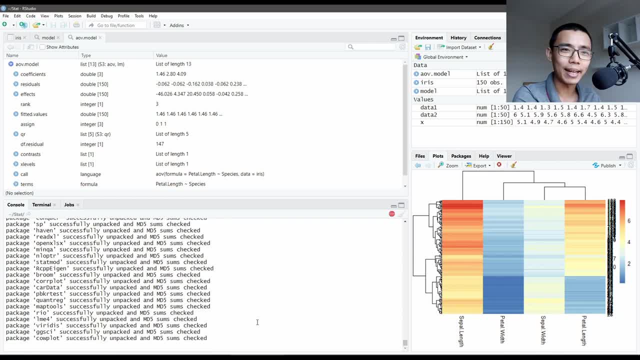 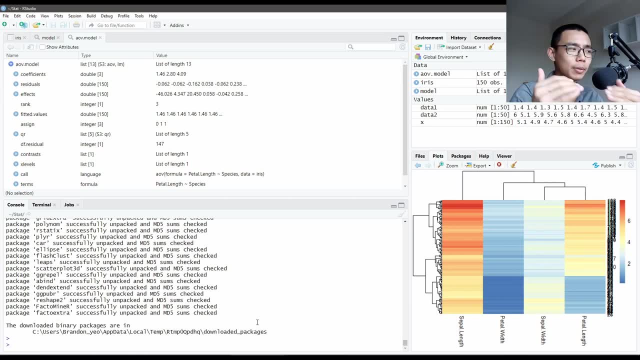 so many packages because they're actually dependencies. When they code one of the package, it depends on multiple. multiple package There's multiple simpler package and they will actually install them together. So that's why you get so many things getting installed on your computer and sometimes it's bigger. 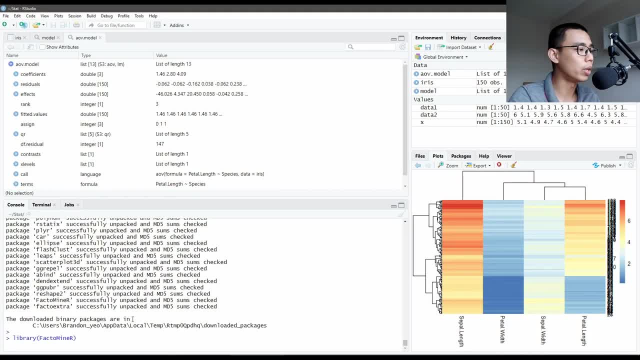 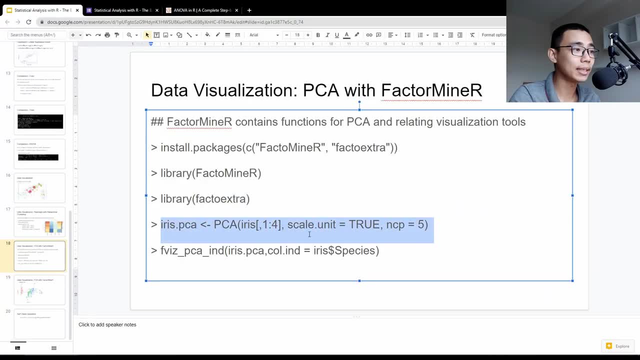 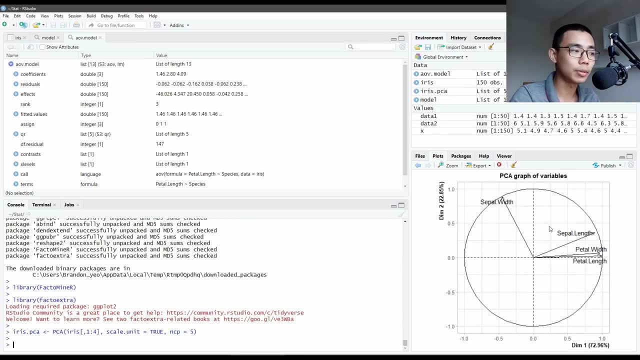 and sometimes it's smaller, it depends. Okay, Let's load the library into your environment and we can run our PCA analysis, which we assign to another new object called irisPCA, And it will actually show you a PCA graph of the variable. 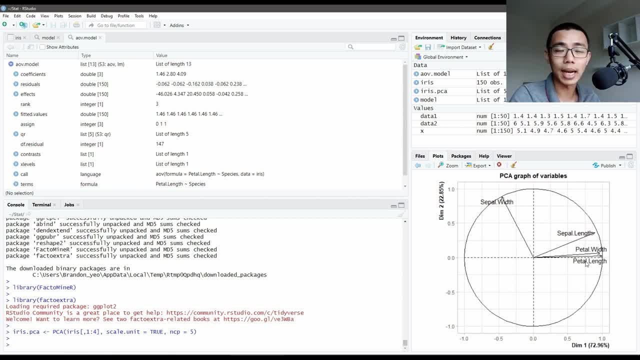 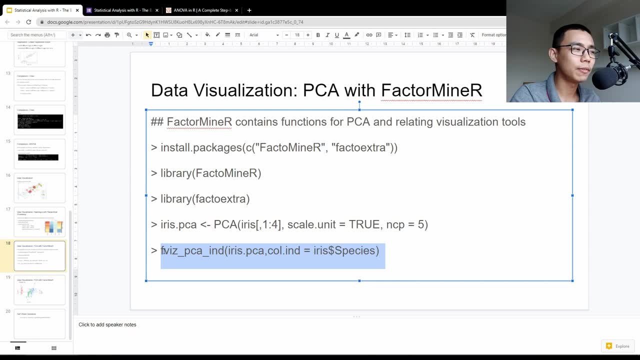 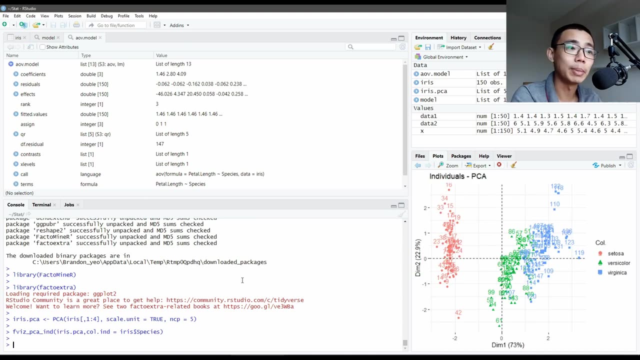 And yeah, you can see that simple width is very far away from the other three columns And you can also try to find that. what is that called F base? PCA, individual means to want to plot individual flowers as the individual points and we can color them based on the species. 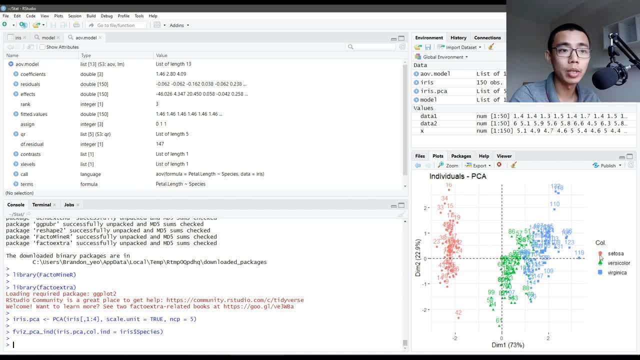 So we can actually see that, based on dimensional one and dimensional two, versicolor and verginga are slightly closer to each other in terms of their flower patterns, While setosa is actually quite far away from the other two species, So it's very easy to separate out setosa.